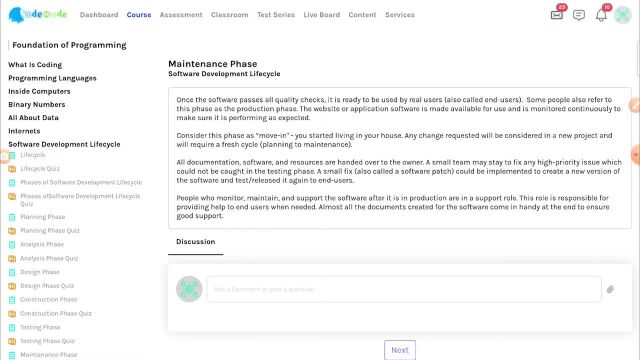 if you are watching on YouTube For complete course and related coding practice, go to our platform, mycodemodeus. Let's begin: Once software passes all the quality checks- which also means all the bugs or defects identified by the quality engineers- are addressed, or 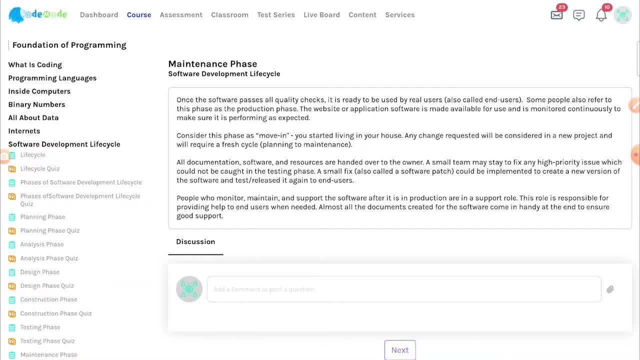 fixed by software developers and retested software is ready to be released. What it means is it is ready to be used by the end user. In this case, when I talk about codemode, the software is ready to be used by students like you or teachers like me or some other. 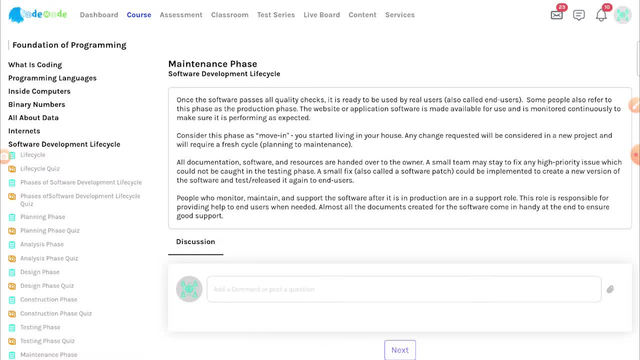 teachers. Some people also refer this as a production phase. The website or the application is continuously monitored, especially in the beginning when a software is released, And it is monitored to make sure that all the functionality or the features are working as expected. Consider this phase as a move in when it comes to with respect to the example. 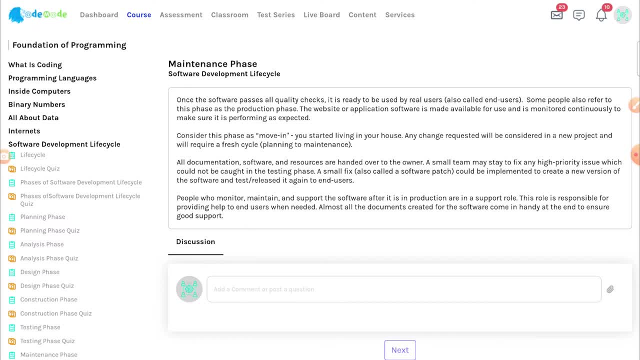 I was giving you about the house construction. The house is handed over to you. you, as an owner, You start living in the home. You may find some issues here and there which you may call the contractor and tell him or her to fix it. That is what we refer as a support. 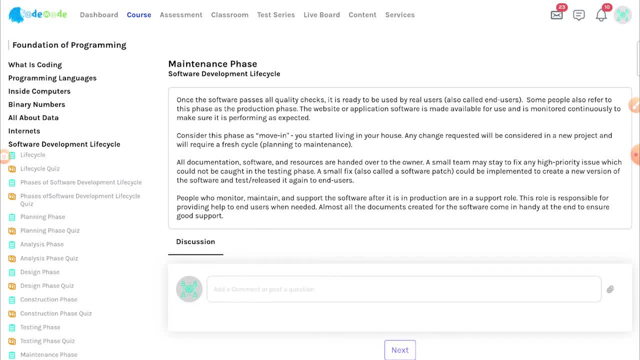 phase or warranty phase. So usually you have a certain period in which anything that goes wrong in the software, anything that was not caught during your testing phase, may still be fixed in this phase. All the documentation, the software, all the resources like the. 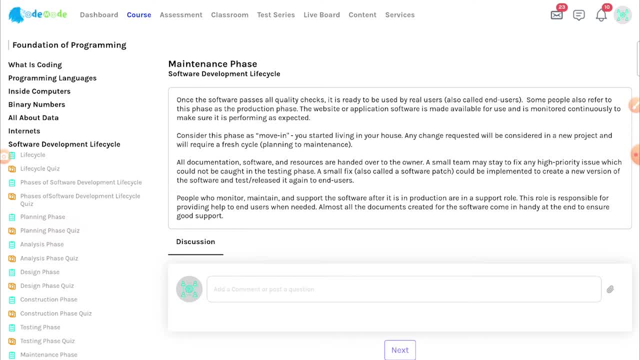 laptops and everything are handed back to the owner. A small team may still be available to fix any high priority defects that were identified by the end user And those you know, those soft. those issues would be resolved and released on top of the main software. 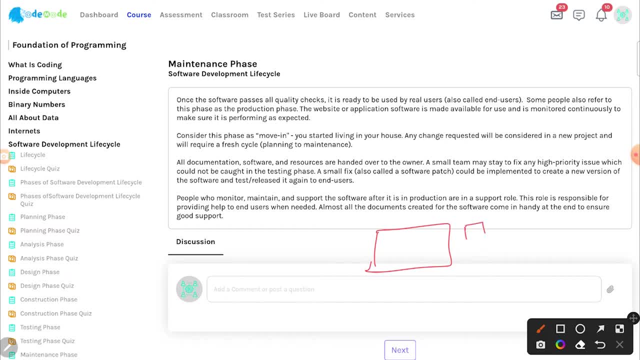 So if this is the main software- let's say this is the main software- it is possible that you will release a set of like five bugs that you addressed as part of what we call this as a patch and you release the patch. That means you apply this patch on the main software and change the code, This patch.